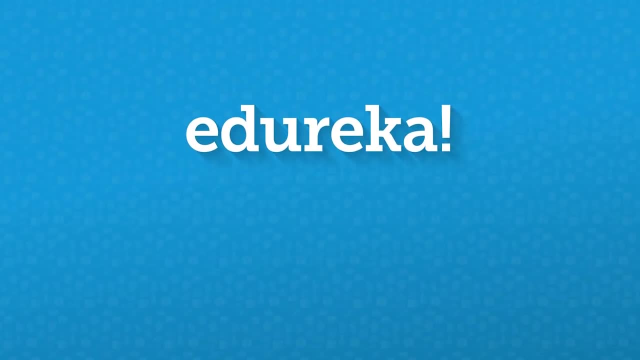 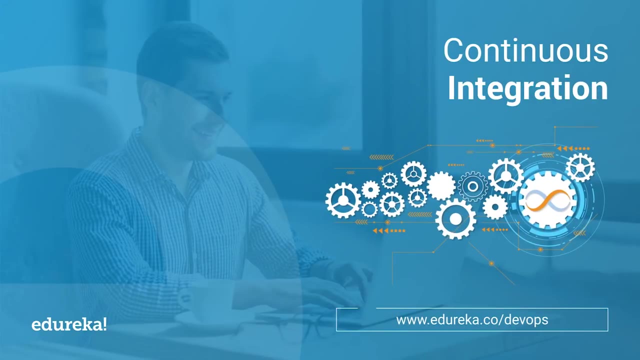 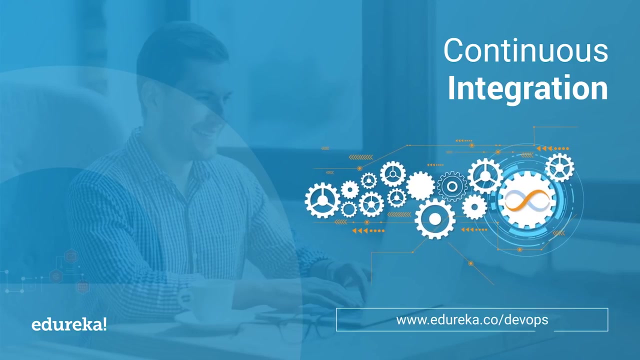 Continuous integration is a practice that helps developers deliver better software in a more reliable and a predictable manner. In this video, you will first see how developers face problems while writing, testing and delivering softwares to their end users So well, once you understand. 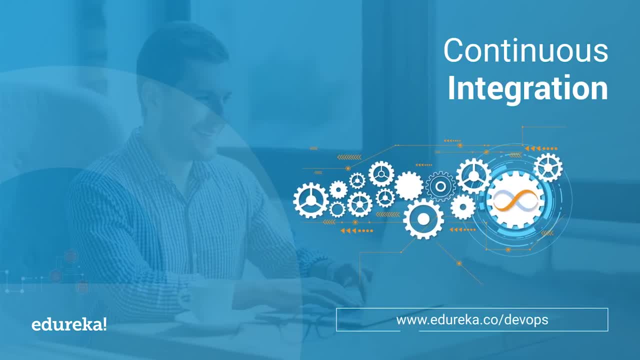 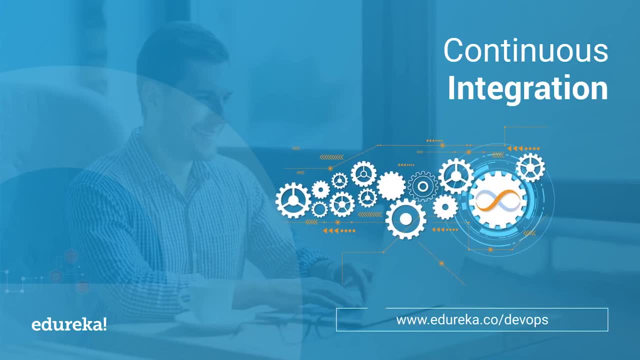 these problems, you'll understand that these problems were solved by none other than continuous integration. So, hello everyone. This is Sahithi, on behalf of Edureka, and I welcome you to this session on continuous integration. So thank you, all the attendees, for joining in today's session. 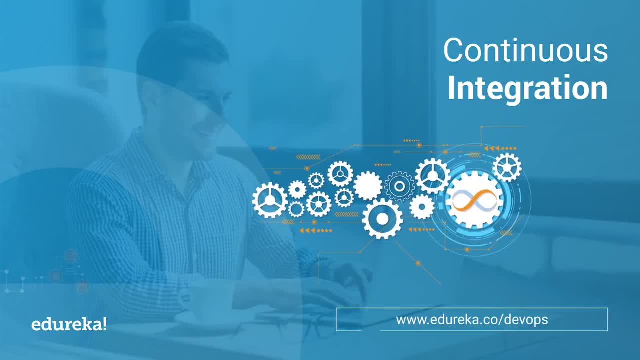 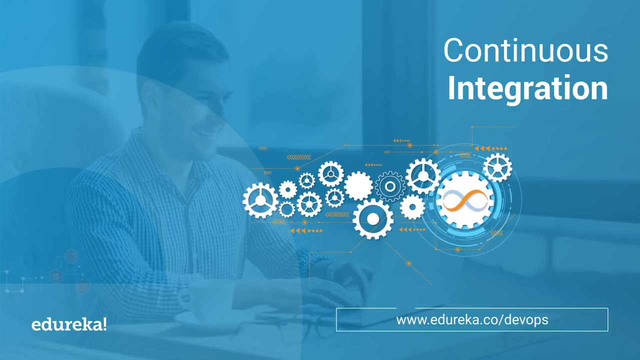 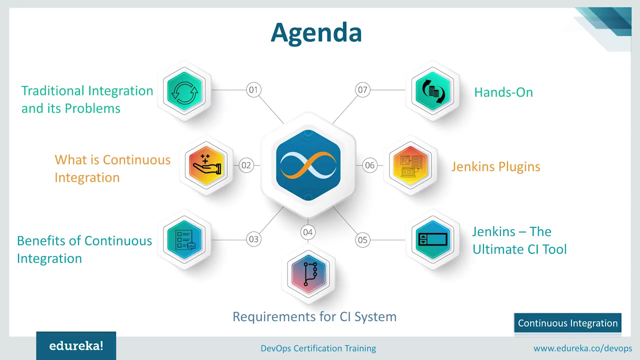 Before we get started, all of you just give me a quick confirmation on the chat window whether I'm audible or not. Okay, I've got many yeses, So that's great. So now let's get started with the session. So, without wasting any further time, let's look into the topics for today's session. We'll start. 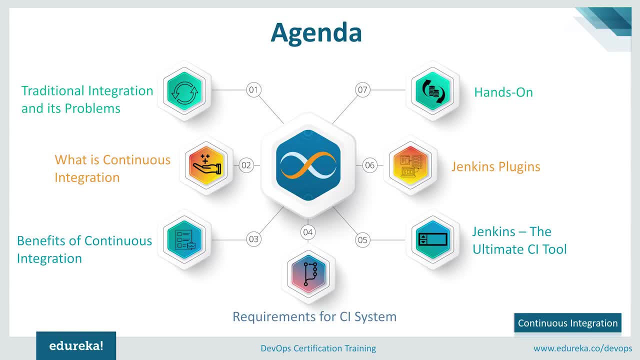 today's session by understanding what was traditional integration and its problems. Then we'll understand what is continuous integration and look into the benefits of continuous integration. After you understand the benefits of continuous integration, you'll understand the requirements for continuous integration system and then we'll discuss the ultimate tool for continuous integration. 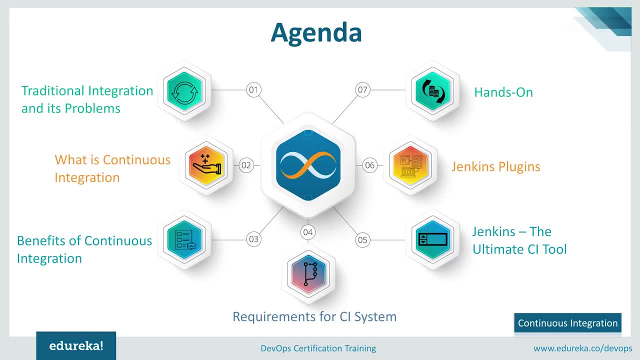 that is, Jenkins. Once we brief about Jenkins, will discuss more about Jenkins plugins And then, finally, we will move on to a hands-on part where we will perform continuous integration with the help of tool Jenkins. All right, guys, So is the agenda clear to everyone? Okay, so that's. 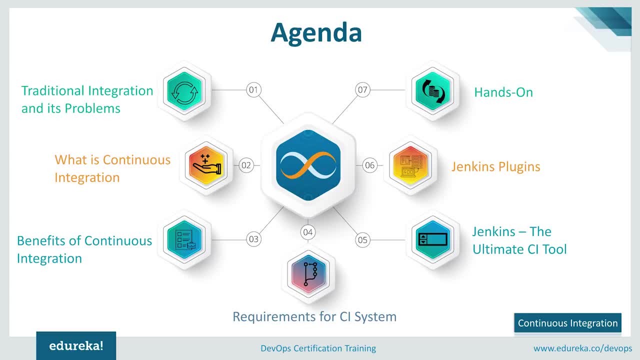 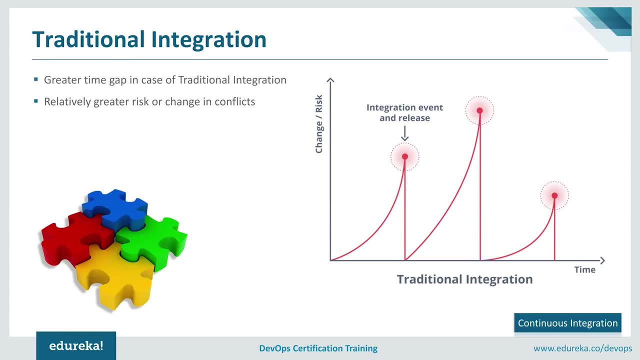 great. So now let's get started with the first topic for today's session, That is, traditional integration and traditional integration. Each developer gets a copy of the code from the central repository with the standard integration. So let's get started with the first topic for today's session. 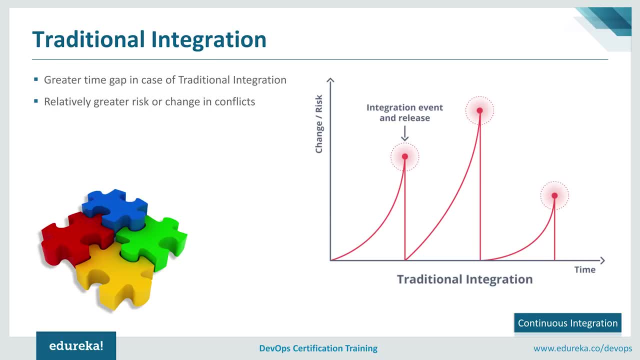 Let's get started with the first topic for today's session, That is, traditional integration. and traditional starting point is none other than the latest stable version of the application. Now all the developers begin at the same starting point and work on adding new features or fixing bugs. 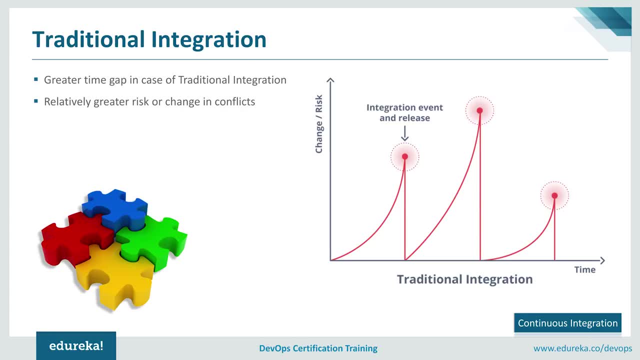 So each and every developer makes a progress by working in a team or on their own. Now, what I'm talking about is each developer is trying to add new feature or is fixing any bug, So all the developers are working simultaneously on the same code. 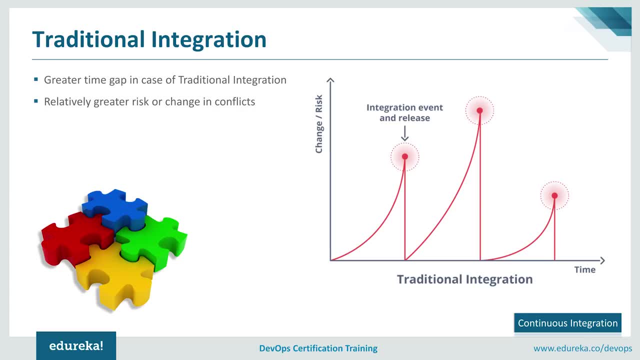 They add or change classes, methods and functions and shape the codes to meet their needs and eventually they complete the task they were assigned to do. so each and every developer performs these actions and they keep changing the code to fulfill the task that they were assigned to. so, if we just take a step back, 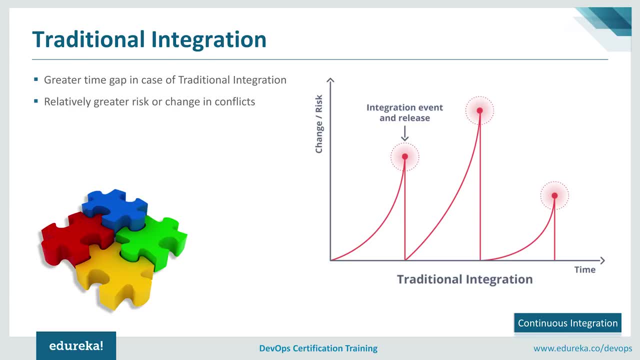 and look at the entire project, we can see that all the developers working on the project are changing the context for the other developers, as they're working on the same source code, right? So suppose you consider a team of five developers, So each one of them is changing the code again. 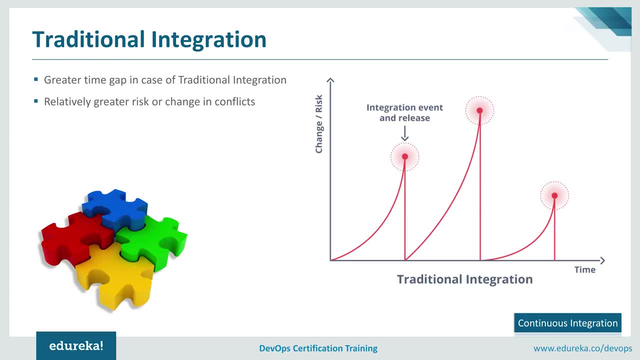 and again to just fulfill their features. now, as teams finish their tasks, they copy the code to the central repository. Now there are two scenarios that can happen at this point. either the code in the central repository is unchanged or the code in the central repository is changed right. 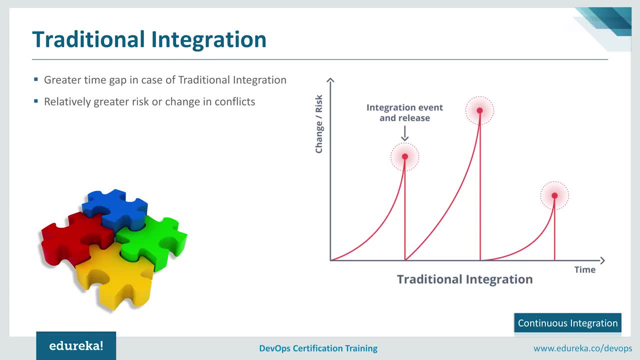 So, considering these two scenarios, you can obviously see that there's a conflict in the source code present with all the developers. So nobody has the same source code. if developer is working on feature a, then he has a particular code and that code is not present. 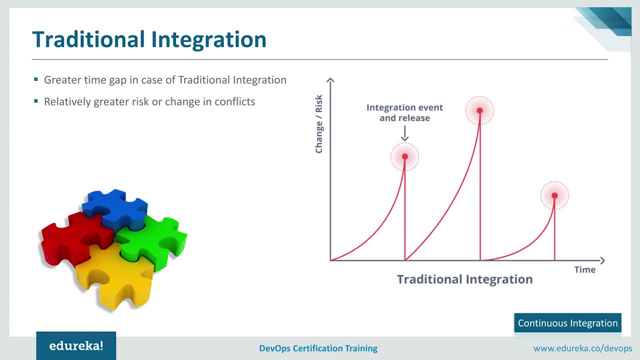 with developer B at that particular instant right. So now, as you can see that this created a lot of confusion for handling the source code right. So what are the main factors that can make these problems escalate? So suppose if there's a big team working on a project. 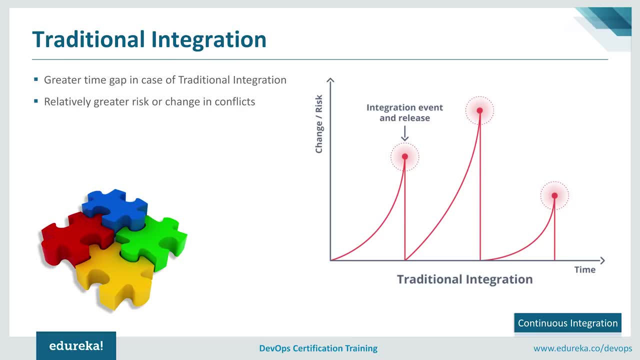 then integrating the code of each and every developer working on the team becomes difficult. Also, the amount of time passed since the developer got the latest version of the code from central repository is very much increased. by this I mean that suppose at one instance developer a has some code. 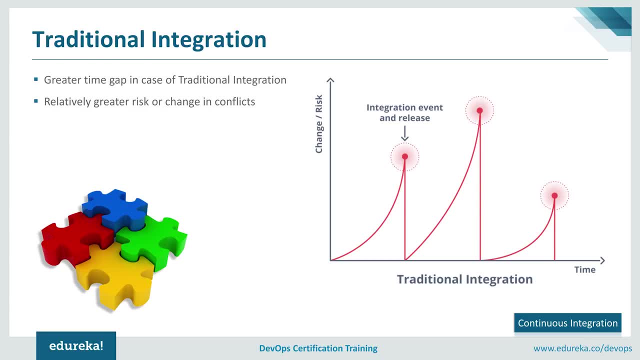 with him and there are so many few commits already made right. So by the time the developer a again gets the code, the time lapse between developers, a code and the rest of the team is much increased. now that I've told you What traditional integration is, let me explain you further. 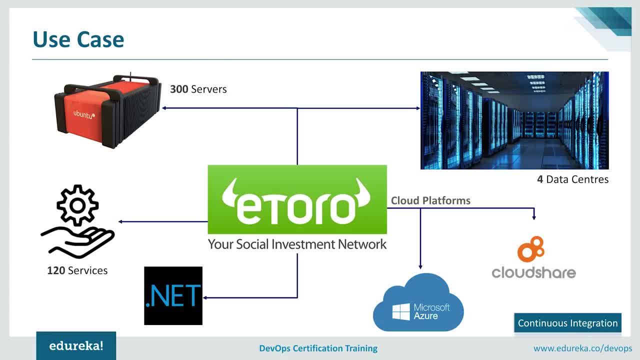 with the help of a use case of a company. So we have a company known as Itoro. Itoro is the leading social trading and an investment network company. This company has 120 services, around 300 servers working on Ubuntu. It has four data centers and two cloud platforms. 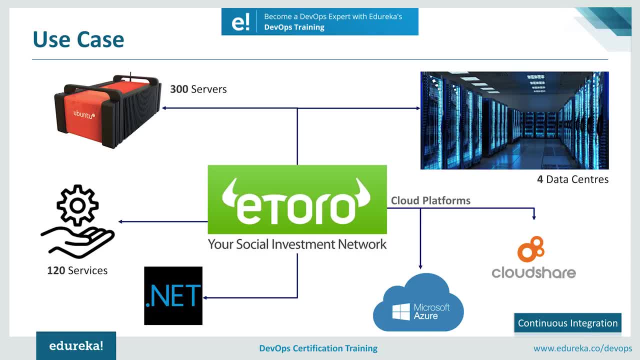 that is, cloud share and Microsoft Azure, And finally, it also uses the dotnet languages for implementing their codes. Now, as you can see that this company works on a large-scale industry, There were many problems faced by the developers, So now let's look into the problems. 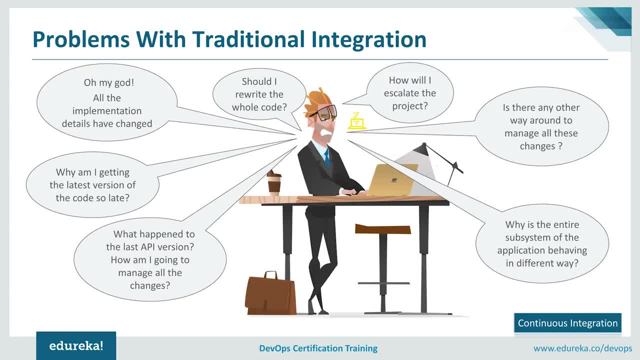 that were faced by the developers. So when you see the problems with this company, the major problems faced by the developers, where they could not build the applications easily, They had to manually deploy all their applications, They lacked uniformity. that is suppose 10 developers. 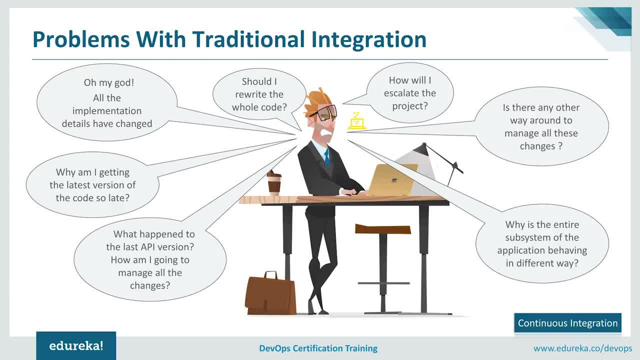 were working all the 10 lakhs uniformity between each other. That is because they were working on different operating system environments and they had to configure it separately to get uniformity between each other. also, they lacked performance issues, which is like the main trademark for any company. 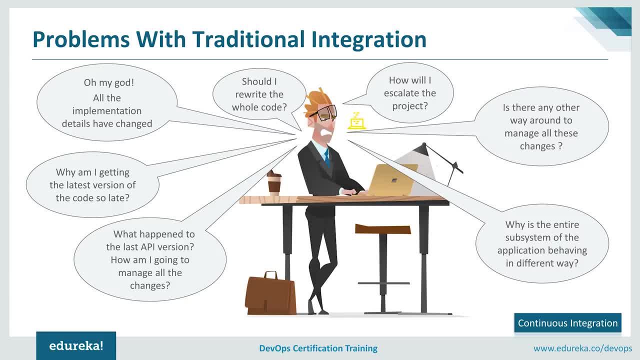 because any company in the market needs to have a good performance range and they had a really slow performance range. And finally, when the complete team was trying to integrate their codes, then they found that they had lack of security between while they were integrating their codes. 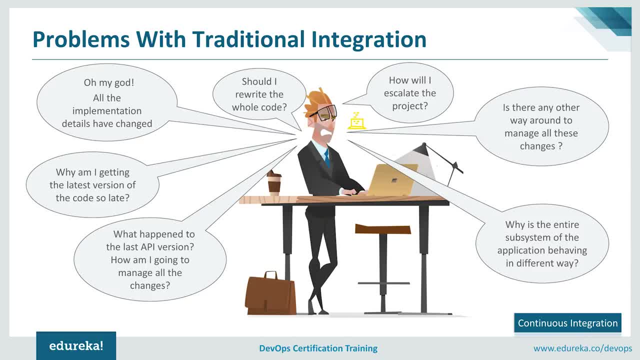 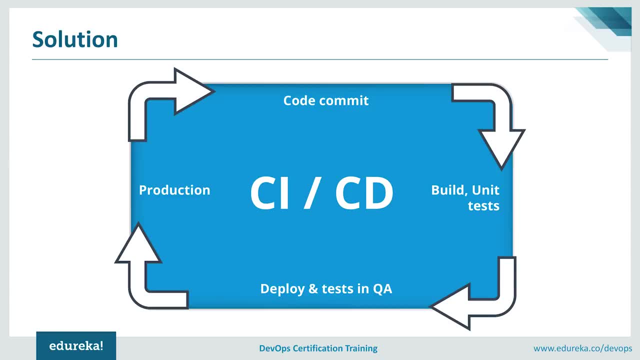 These were some of the major issues that the company was facing. Now, what was the solution for this? How could the developers overcome these problems? Well, the answer to this problem was continuous integration. So what the developers did was they created a continuous integration and a continuous delivery pipeline. 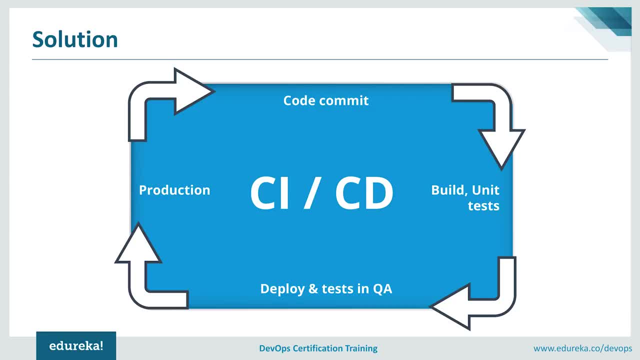 which automatically built, tested and deployed their application onto various servers whenever a new update was committed. So, as I told before, they had 300 servers. So with the CI CD pipeline they could automatically build, test and deploy their application into any number of servers they wanted whenever the update was committed. 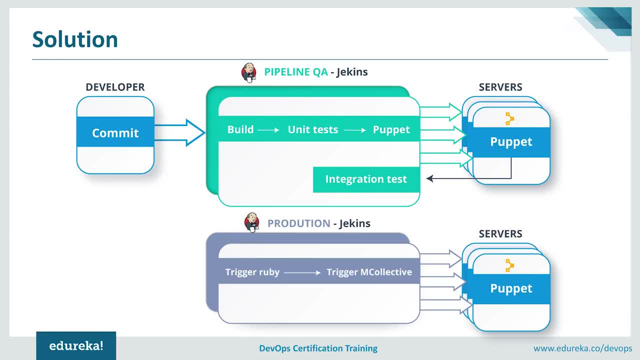 So, as I was telling you, how did they create the continuous integration pipeline? Well, to create this pipeline, they use the Jenkins tool, which automatically build the application and perform unit test. that is nothing but the user acceptance test. after that, they integrated puppet with Jenkins. 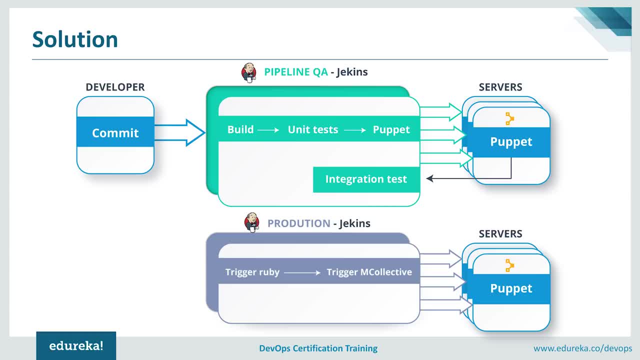 and used to configure the environment and deploy the applications to their servers. this automated the complete process by removing all the repetitive manual task and streamline the environment that does it maintain the uniformity between all the developers working in the company. So this solve the major problem now. 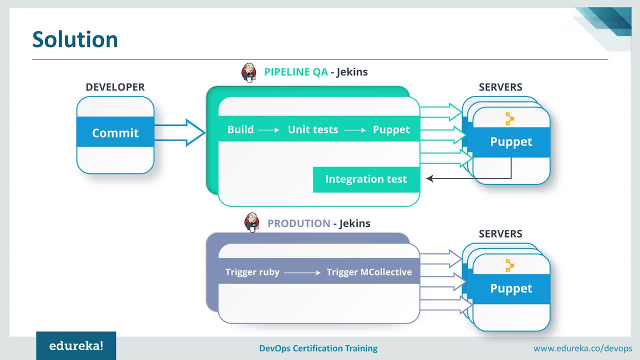 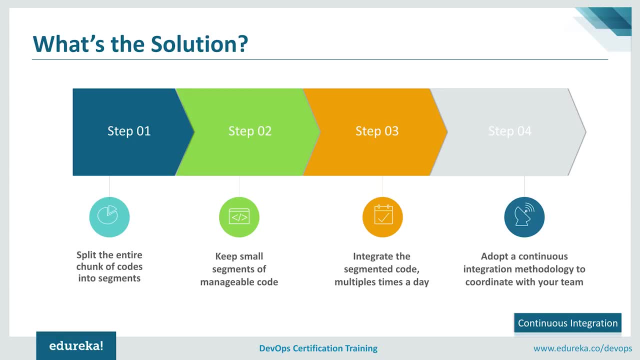 as I was telling you about continuous integration pipeline, continuous delivery pipeline. Now, what exactly was this continuous integration pipeline? Now, before I tell you what exactly is the continuous integration, Let me tell you how it is done. You have to split the entire chunk of codes. 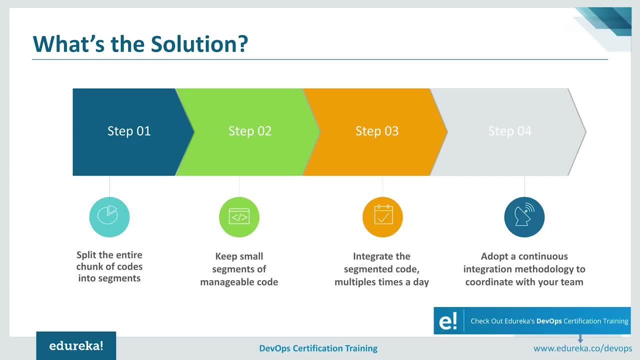 into segments first. then you have to keep small segments of this manageable code after you make the changes required. You then have to integrate the segmented code like multiple times per day, so that your everybody has that code, and then finally adopt the continuous integration methodology to coordinate with your team. 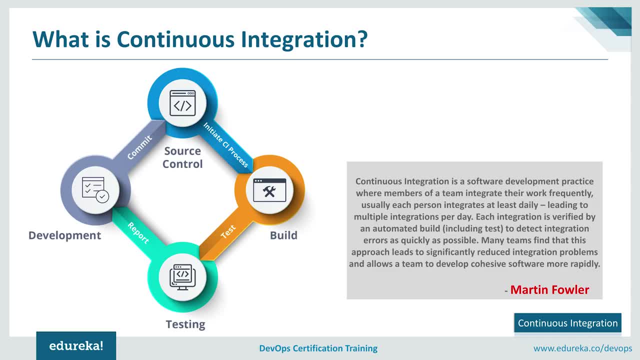 Now, what exactly is this continuous integration? So, according to Martin Fowler's formulation, continuous integration is a software development practice where members of the team integrate their work frequently. Usually, each person integrates at least daily, leading to multiple integrations per day. Each integration is verified by an automated build. 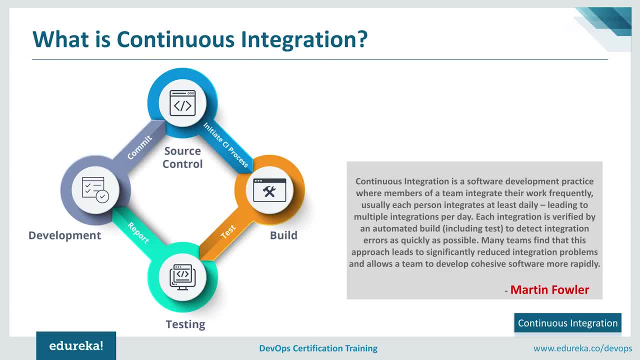 to detect integration errors as quickly as possible. many teams find that this approach leads to a significantly reduced integration problems and thus it allows a team to develop cohesive software more rapidly. Now let me explain you this definition in simpler terms. continuous integration is nothing but the practice of continuously integrating. 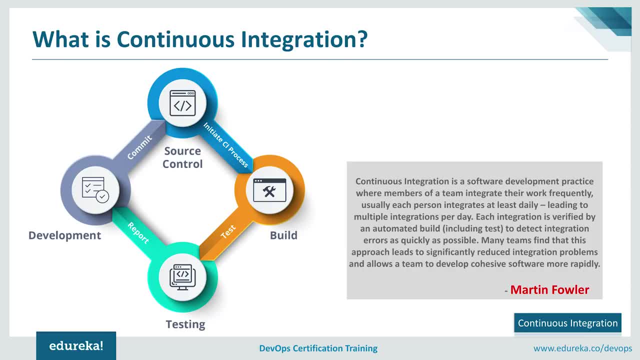 the changes made to the project and then testing them accordingly, at least on a daily basis or like more frequently. now, automating your build, test and deploy processes can elevate many problems commonly happening on projects now. in such situations, having a reliable method of integrating changes more frequently ensures 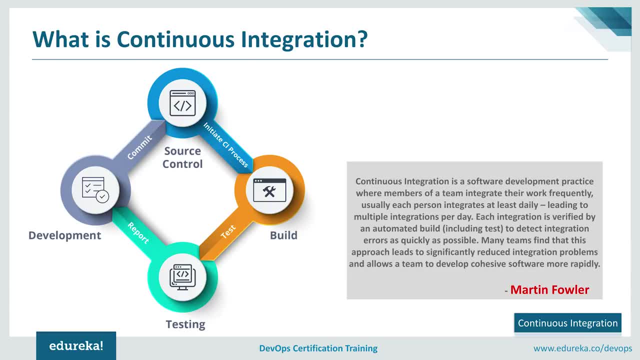 that these errors can be found sooner than later, so that all the problems are solved before anything major happen. So continuous integration solves the errors very soon and also helps in integrating all the source codes of all the developers and makes changes together. So now that you've understood what continuous integration is. 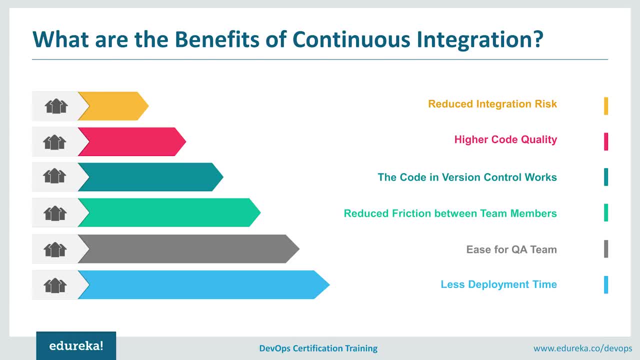 Let me tell you the benefits of continuous integration. So, starting with the first benefit, the first benefit we have on the list is continuous integration offers reduced integration Risk. now, when I talk about reduced integration risk, often working on projects means like multiple people's are working. 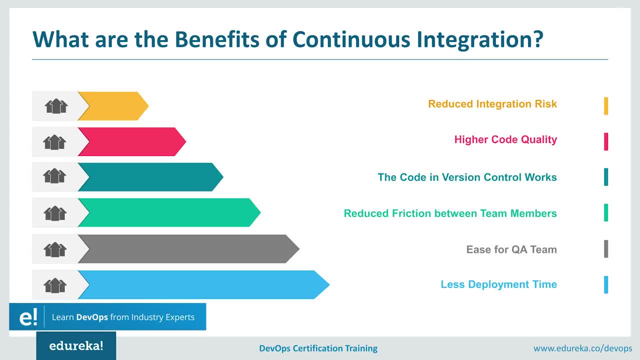 on separate tasks or parts of the code, as I mentioned before. So suppose a team is building an application and that particular team has 10 developers, So each and every developer would be responsible for some of the other functionality of that particular application. now, the more the people, the risk is the integration that's. 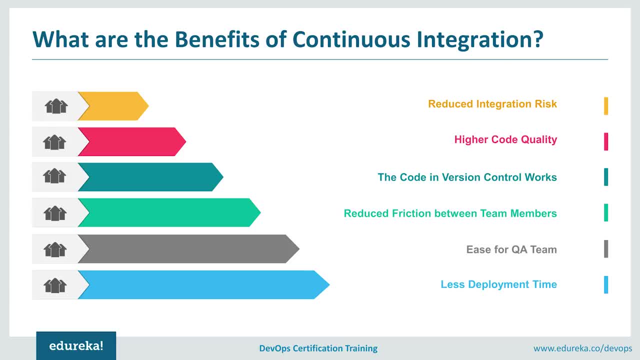 because there's a lot amount of code and each developer has his own copy of the source code with the new implemented change. So now, depending upon how bad the problem is or how large the team is, debugging and solving those issues can be painful and can potentially mean a lot of changes. 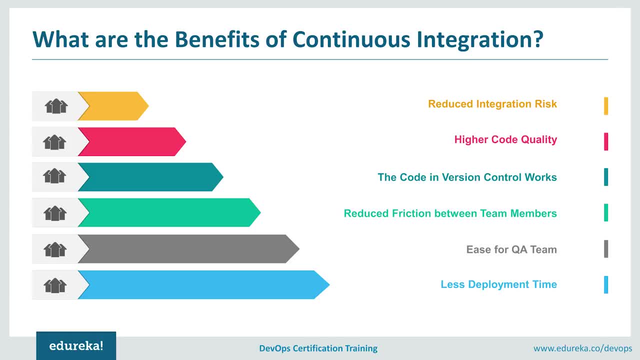 to the code. So when you integrate all the changes made by all the developers into a single code, then it could need a lot of debugging and could also be a time-consuming work. now, integrating daily, or even more frequently, can help developers to reduce these kind of problems to a minimum level. 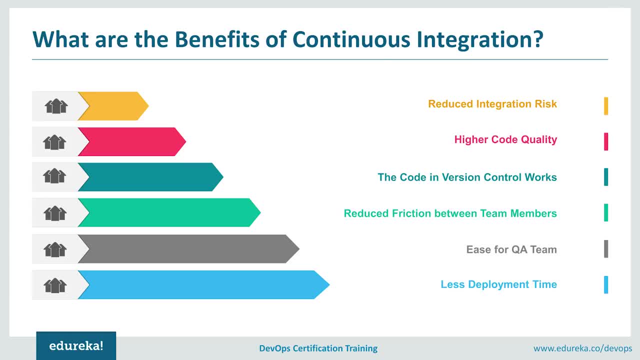 so that they do not have to debug at a large extent. now, that was the first benefit, guys. now moving on, the next benefit We have is continuous integration offers higher quality code. in continuous integration, You don't have to worry about the problems and you just have to focus more on the functionality of the code. 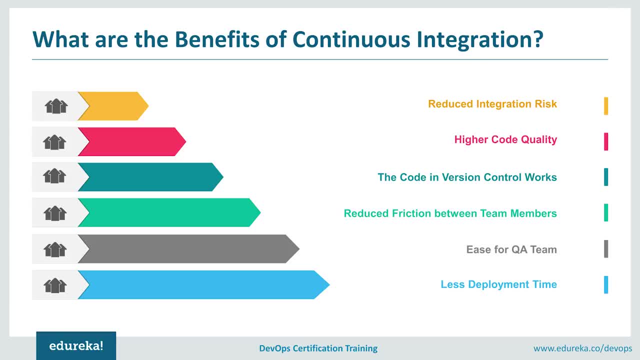 So obviously, when you focus more about the functionality of the code, it results in higher quality problems And products. next, if you use continuous integration, you will observe that if you come at something that breaks the build, you and your team will get the notice immediately and then the problem is fixed. then. 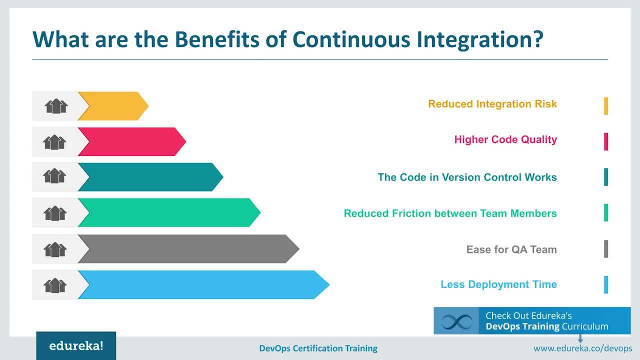 and there, before anybody else pulls that broken code from the central repository. What I'm trying to say is suppose a developer comments a build onto the version control system and there's some error in it, He will be immediately notice that there's some problem with the code and he should immediately fix it. 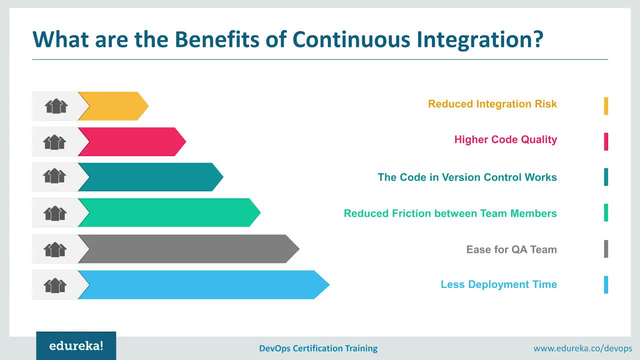 before anybody He else pulls that code. so you can just say that the code and the version control works to help people integrate much better. after that, we have continuous integration offering reduced friction between the team members. So, as it is evident that the continuous integration system is an impartial system, 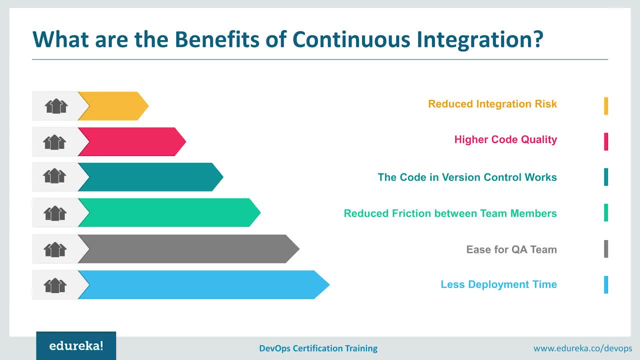 That is, it does not offer partiality to anybody. So if there is any mistake, then that mistake has to be solved. If there's any bug, then it has to be debug. There's no option left in such situations. Offers reduce friction between the team members. 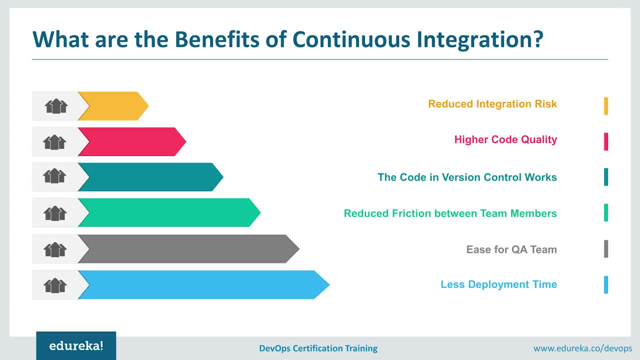 because they know that if there's some problem, they have to solve it without fighting with each other. Also, having different versions and bills of the code helps to isolate and trace bugs efficiently, which makes the work easy for the quality assurance team. So suppose they have to identify any particular bug. 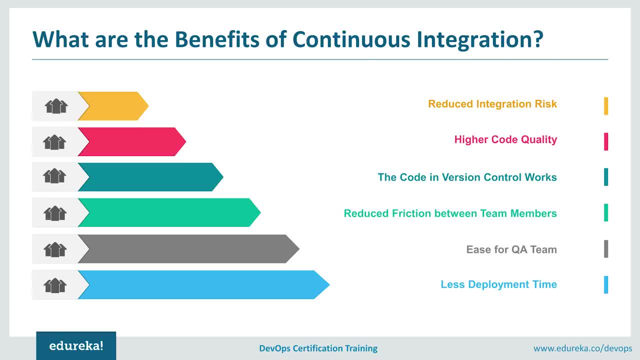 They know how to trace that particular bug and how to solve that bug right. So this makes the life for testing people really easy. and, last but not the least, We have continuous integration, offering less time for deployment, as we all know that deploying projects can be very tedious and time-consuming. 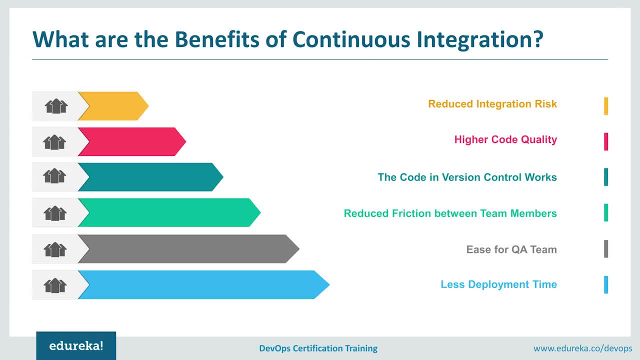 So automating these projects can be really helpful for the complete team. So, guys, that were the benefits for continuous integration. Now that you know what continuous integration is and what are the benefits of continuous integration, It would obviously draw you to an excitement of what are the requirements. 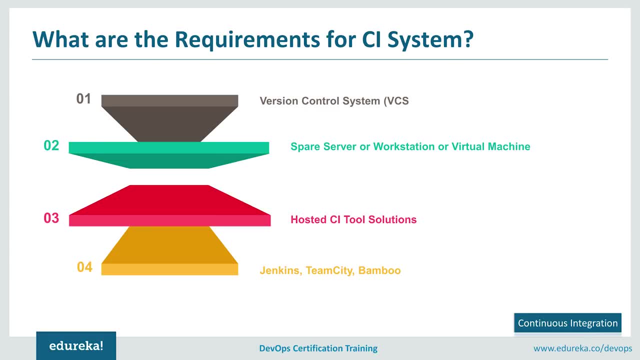 for continuous integration System. so well. there are four basic requirements for the continuous integration system. The first requirement is to have the version control system. Well, version control system provides a reliable method to centralize and preserve changes made to your project over time. 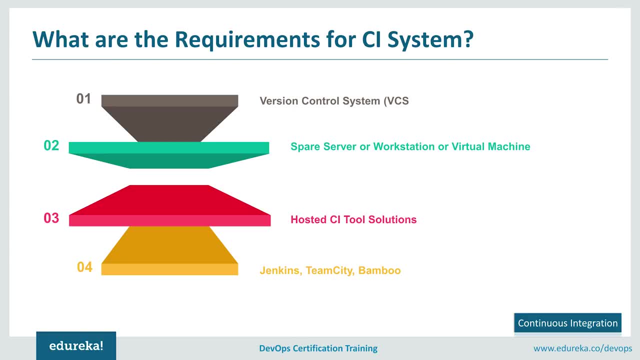 So, as I was mentioning it before, if a team of developers work, then everybody can use this version control system to pull the latest available source code so that they can add their new features, to build any application or to make any change. Also, if you're using on-site Solutions- another requirement- 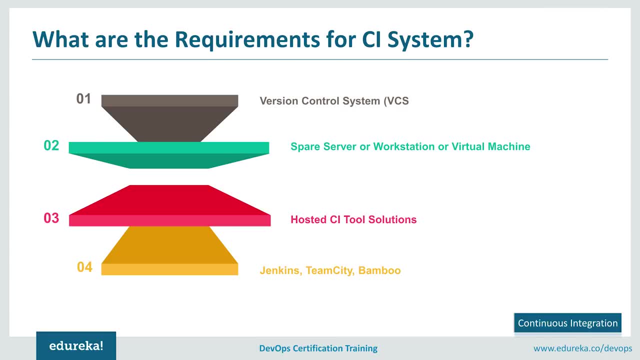 is to have a spare server or a workstation, or at least you should have a virtual machine after that, if you do not want to mess with any other servers or virtual machines. and then, finally, if you opt-in for the self-hosted variance, then you will need to install one. 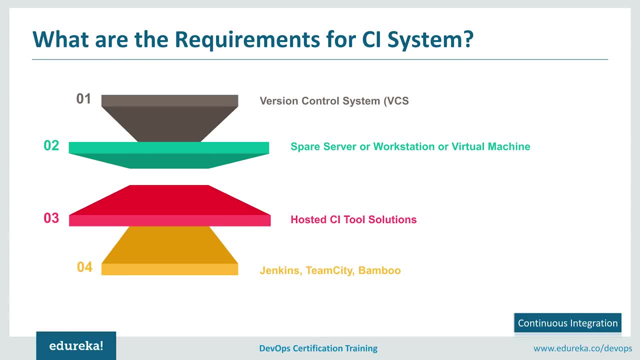 of the available continuous integration tools like Jenkins, Steam City, bamboo, Etc. Right, So, guys, these were the four basic requirements of continuous integration system. Now, as I was telling you in the last point that there are many continuous integration tools, like Jenkins, Steam City, bamboo, Etc. 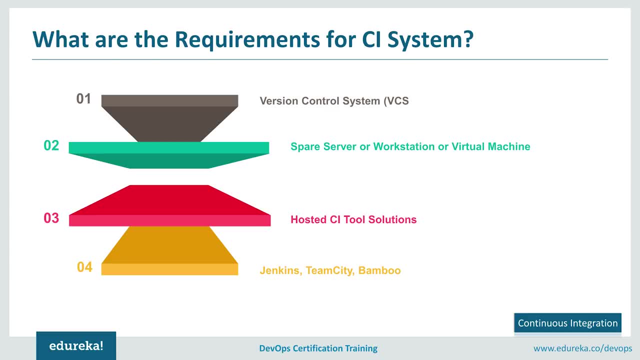 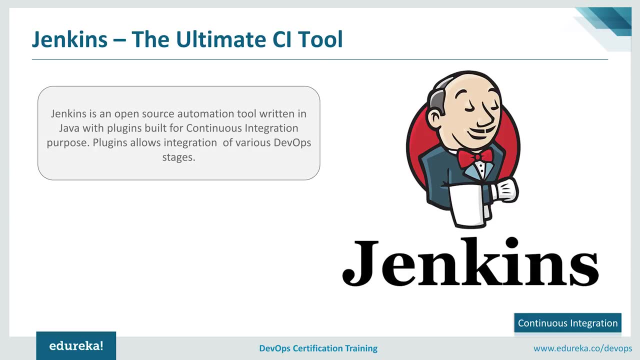 But out of these, in today's Market, the ultimate tool for continuous integration is none other than Jenkins. So let me brief a little bit about Jenkins and then, if you want to deep dive into Jenkins, then you can refer to our what is Jenkins video. 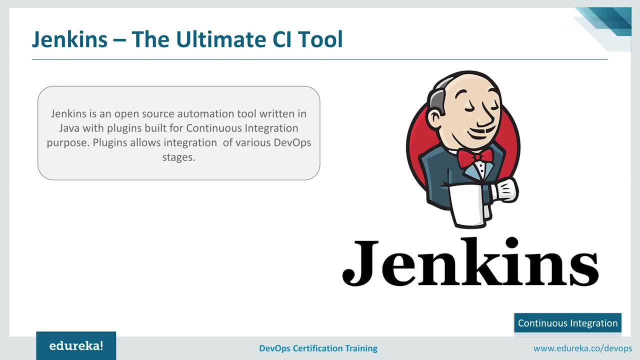 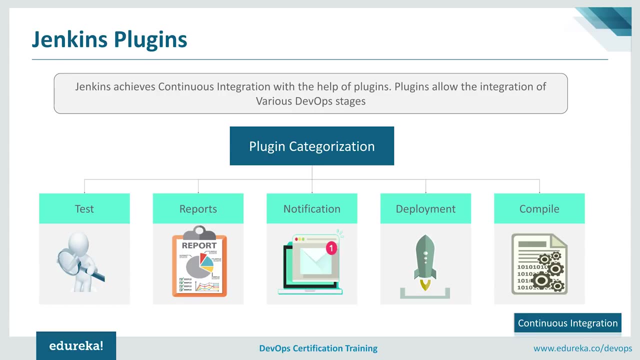 which I'll leave in the description box below. Now let's look into what Jenkins is. So Jenkins is an open-source automation tool written in Java, with plugins built for continuous integration. Well, plugins basically allow the integration of various devops, stages like the continuous development. 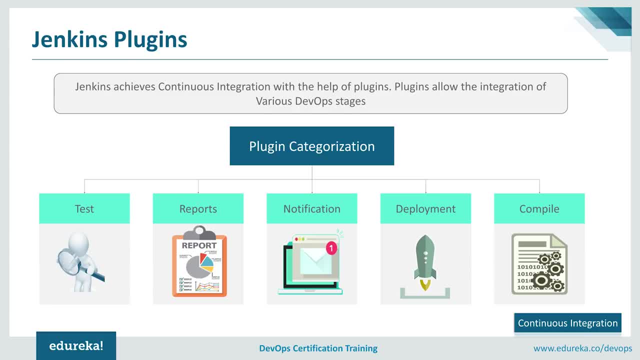 continuous testing, continuous integration itself, continuous deployment and continuous monitoring. So, as it is evident that integration is the heart of the complete devops cycle, So all these stages of devops integrate through Jenkins. So, as I just mentioned about plugins, will Jenkins achieves continuous integration. 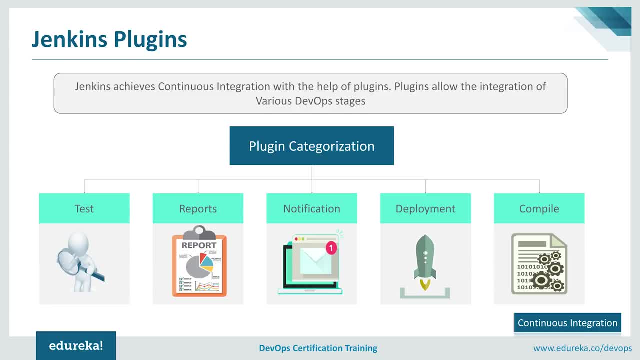 with the help of plugins. now, plugins allow the integration of various devops stages that I just mentioned. So suppose if you want to integrate a particular tool, you just need to install the plug-in for that particular tool. like, for example, if you want to integrate get maven to project HTML publisher. 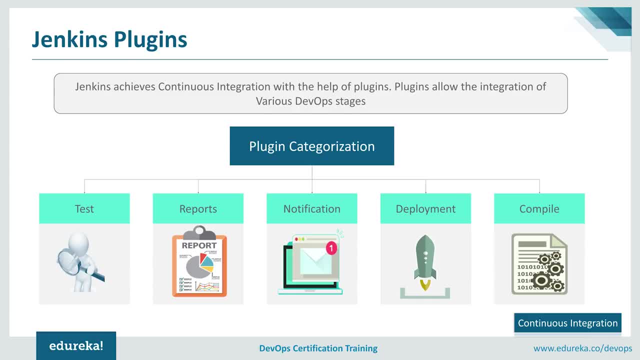 etc. you just need to install that plugins for these particular tool, which I'll be showing you in the hands-on part right now. apart from that, plugins are categorized into various types, like the test plugins, the report plugins, the notification plugins, the deployment plugins and the compiled plugins. 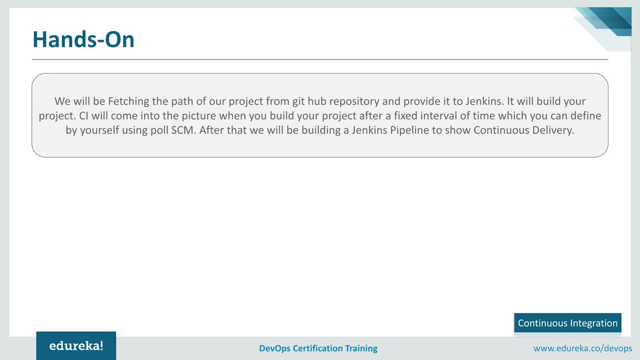 So, guys, that was about continuous integration. So now let's move on with our hands-on part, and our hands-on will be fetching the path of a project from a GitHub repository and then provide it to Jenkins. after that, it will automatically build the project, and then continuous integration will come. 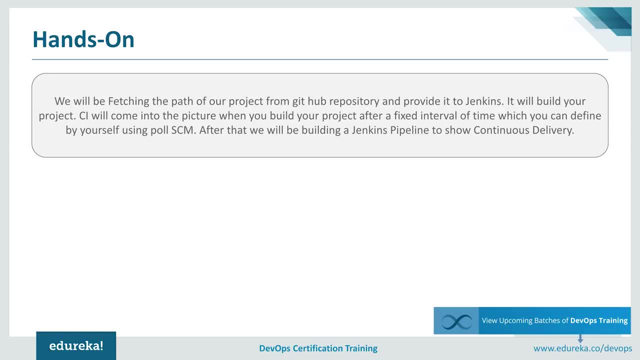 into the picture where we want to build a project after a fixed interval of time which can Define by itself by using the pole SEM, and then finally will build the Jenkins pipeline to show the continuous delivery. All right, So is the problem statement clear to everyone. 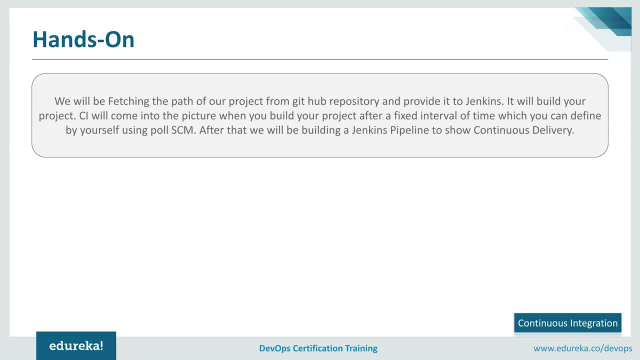 So what we are trying to do is we're going to fetch a path from the GitHub repository and then provide it to Jenkins. after that we will build the project, and then we want the project to be built at a fixed interval of time, again and again by itself, by using pole SEM. 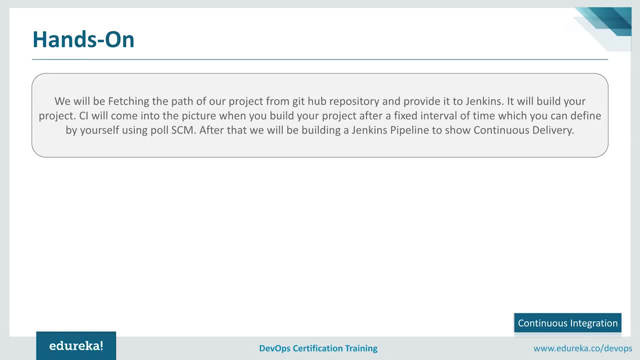 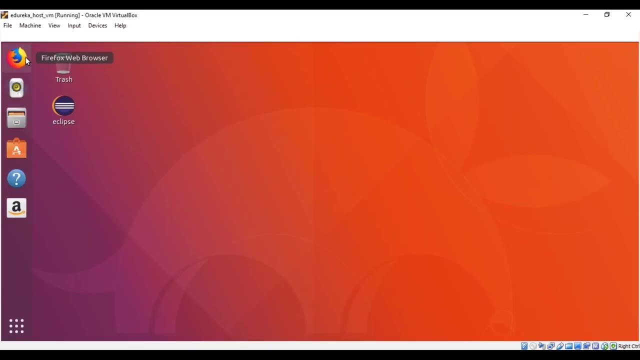 and then, finally, will be building a Jenkins pipeline to show continuous delivery. So now let's get started with the hands-on. So to go to the Jenkins tool, let me go back to my virtual machine and then open the Firefox web browsers so that I can open my Jenkins tool and show you guys. 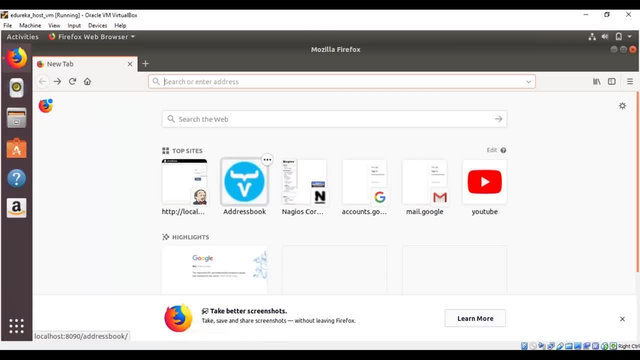 So let me just open my Firefox web browser. So once our web browser is opened up, we have to go to the port where our Jenkins is allocated. right, So I'll go to my local host, port number 8080.. That's where my Jenkins is allocated. 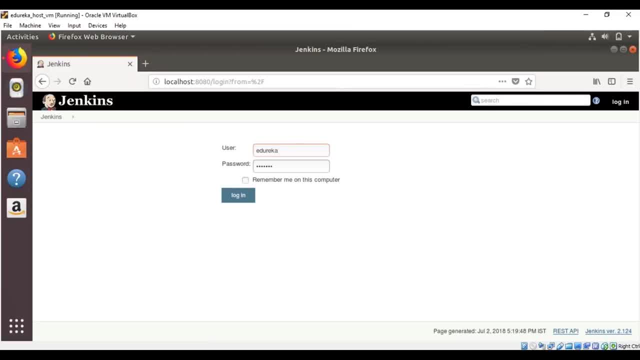 So let me just go to the port And you can see that Jenkins opens up. So now you have to just fill in the login details and then you have to click on login. So I already have my login details filled, So I'll just click on login. 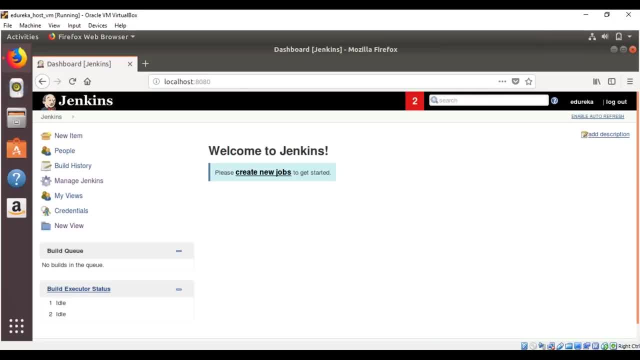 Now, once you log into your Jenkins tool, you can see the dashboard of Jenkins right. So on the left side you have options such as new item, people build history, manage Jenkins, my views, credentials, Etc. And then you have in the main center as welcome to Jenkins. 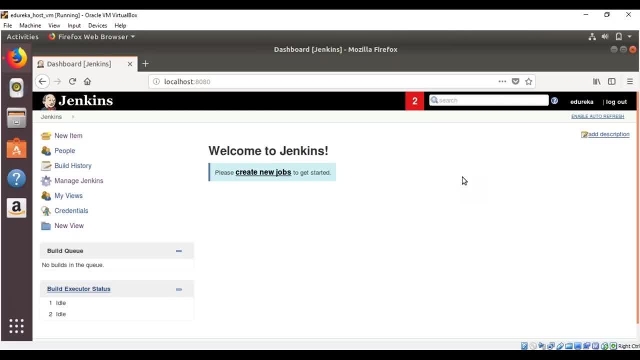 where you can create new jobs to get started right. So if you have to create a new project, you have to click on this option as new item. So let me just click on that Now. once you click on this option, new item. 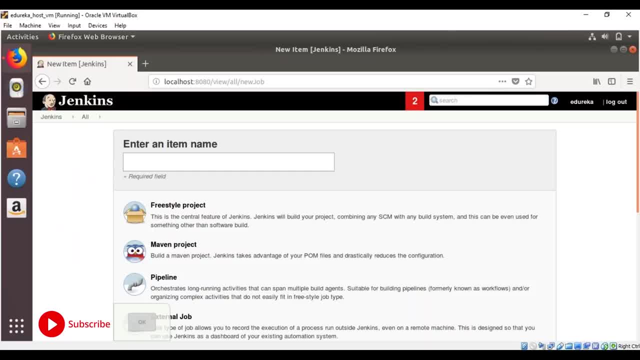 you'll find this page opening up where you have to basically enter your item name. Now, item name is nothing but your job name. Suppose, I put the job name as job one and then I choose the type of project to be- freestyle project. So there are various types of projects that you can choose. 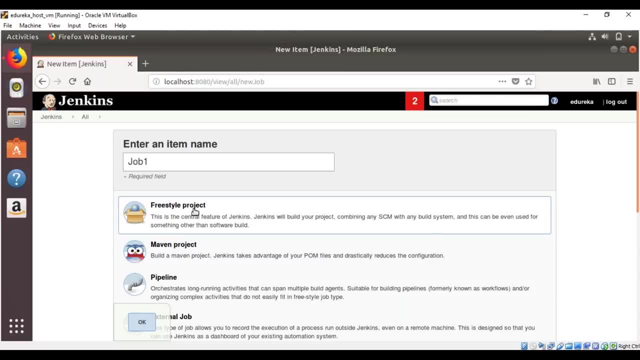 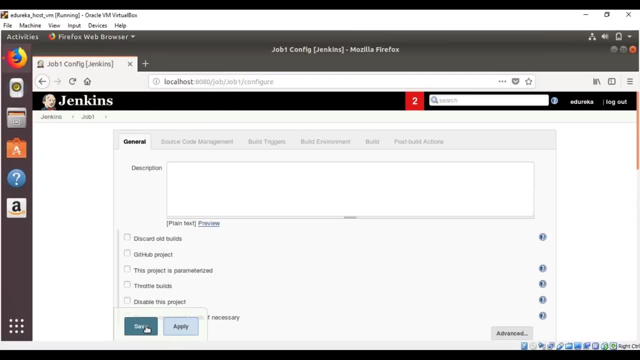 like Maven project, pipeline, external job, freestyle project, Etc. So here I'm choosing freestyle project and then I'll click on ok. Now, once you click on ok, you can see that you have been redirected to another page where you have to fill in the details for job one. 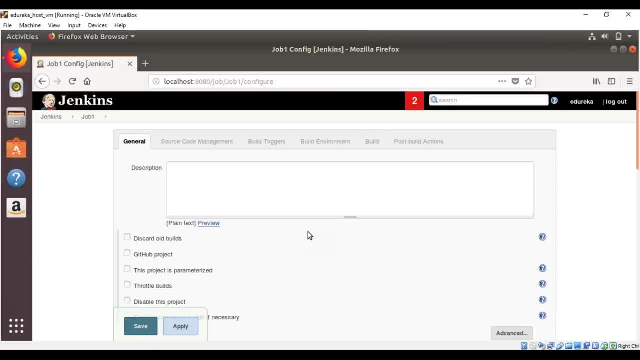 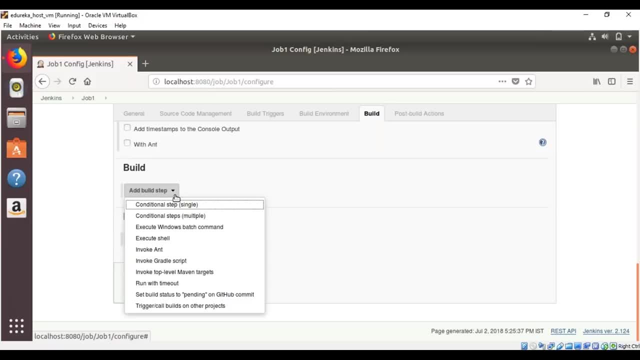 So what you have to do first is you have to go to the option build and then you have to choose the add build step. So you can see in the options of add build step that there are various options present like execute shell invoke and invoke Gradle script, execute Windows batch command and Etc. 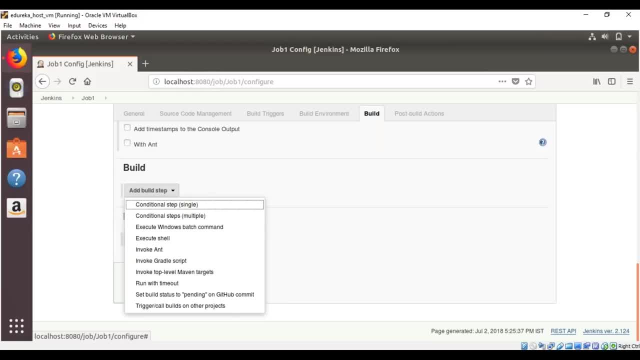 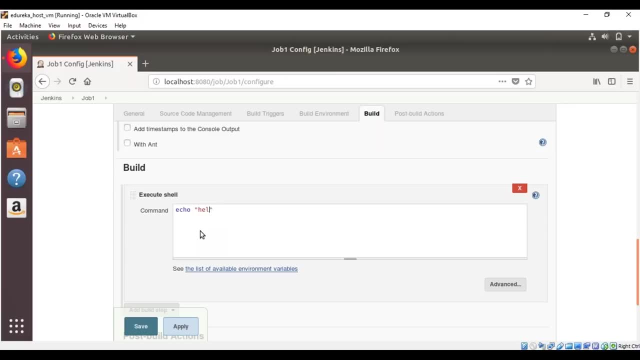 So here we will choose execute shell. So let me just choose execute shell and then in the command I'll just type in eco, hello world. So what this command will do is this will basically print hello world whenever our build is successful. So once this is done, 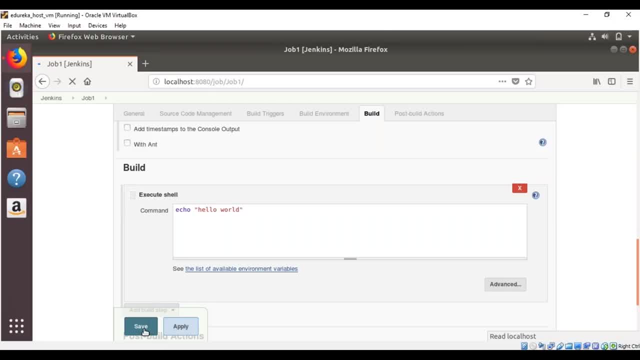 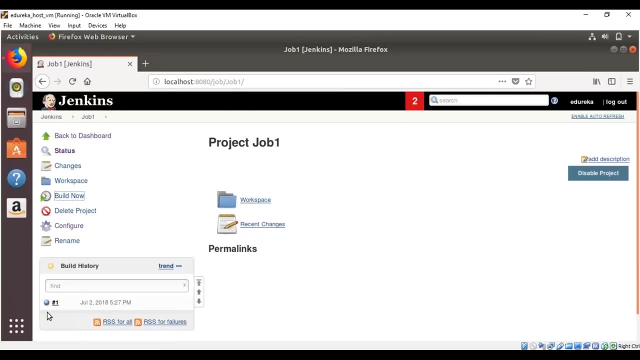 I'll just save this and then now you can see that our job one has been created. Now you have to build your project right, So for that you'll choose the option build now. Now you can see over here that our first build is successfully completed right now. 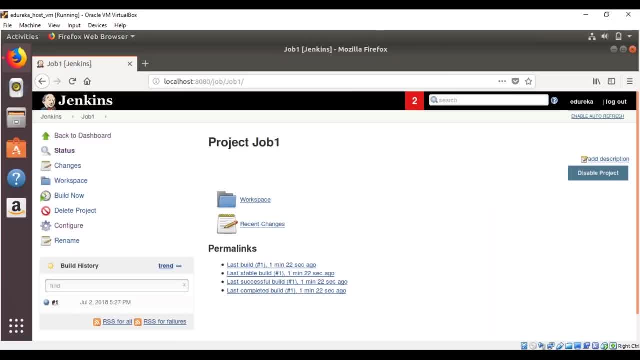 What I want to do is, apart from just using the shell commands, I also want to pull a GitHub repository. So how do I do that? So, to do that, you just have to click on this option, configure, and then, once it opens, you just have to go. 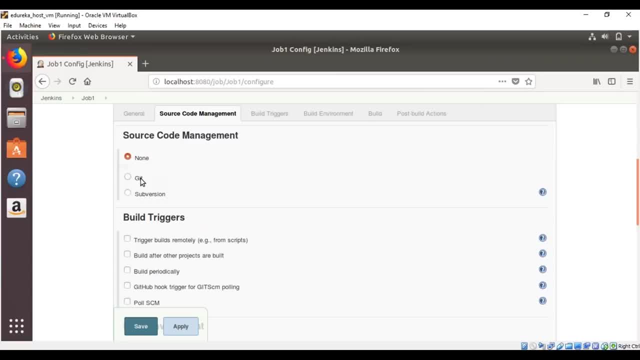 to the option of source code management and then you have to choose your repository type, right? So my repository type is of get, so I'll choose the option get and then I'll mention the repository URL here Now, once you mentioned that GitHub repository. 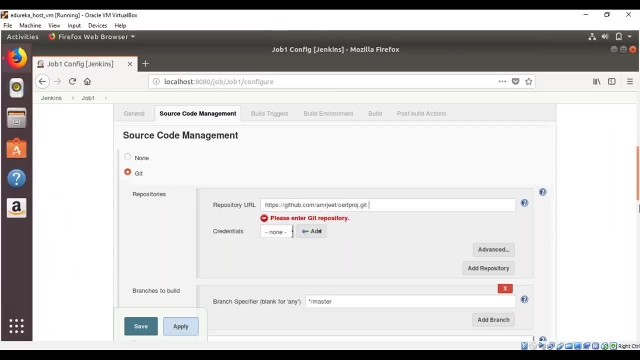 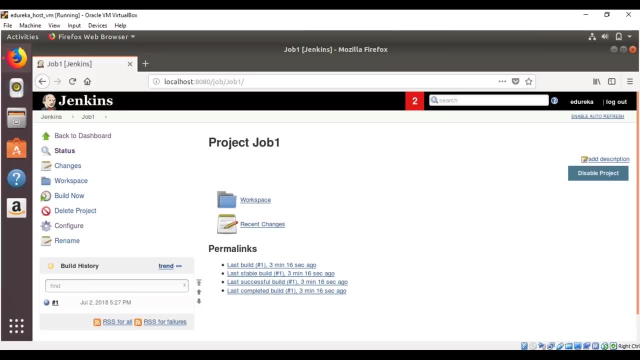 you just have to click on save and then you're done with it. So let me just save this. So you just have mentioned your GitHub repository. You are ready to pull the code. Now, if you want it to work, you again have to build it. 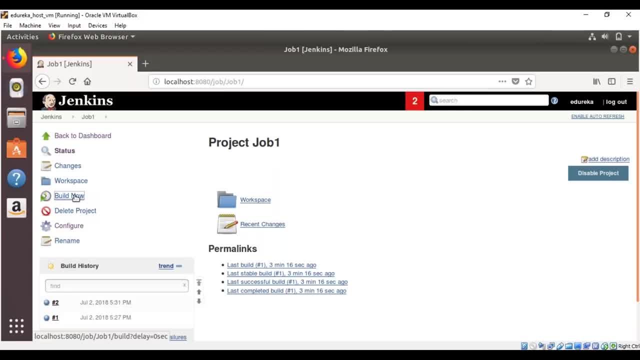 You just have to click on this option build now, and this will automatically build your project. So we just have built a job one now. So now let's just see if it is successful or not. So for that, I just click on this last build over here. 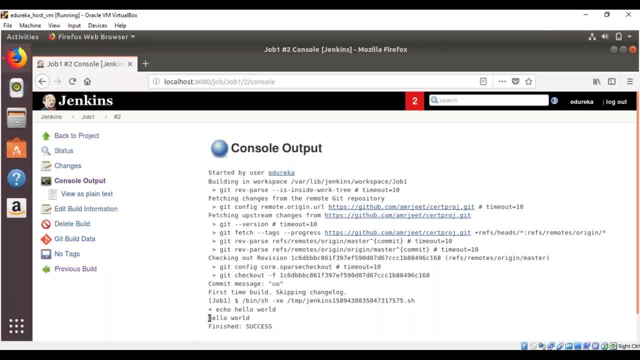 and then check the status so you can see that our hello world has been printed and our build status stands successful. So, guys, that's how you can build your project speed, and you can also pull the code from your GitHub repositories and use shell commands. 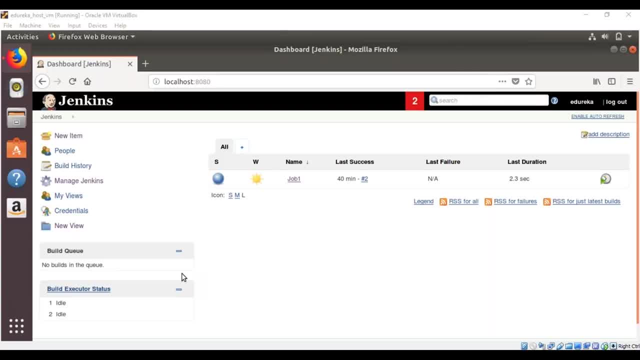 So now that we have seen that a job- one- is built successfully, Now if we want this build to happen again and again at fixed intervals of time, then how do we do it? to do that, Let me just create a new job again and show you how to do that. 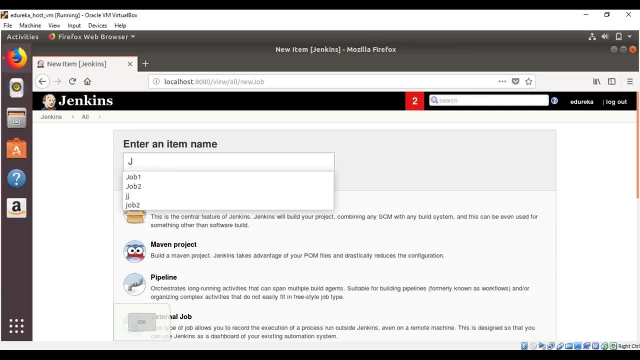 So let me just go to the new item option. So I'll enter the job name as job 2 and then I'll again Choose the project type as freestyle project, right? So once I'm done with that, I'll click on OK and then we are redirected to this page. 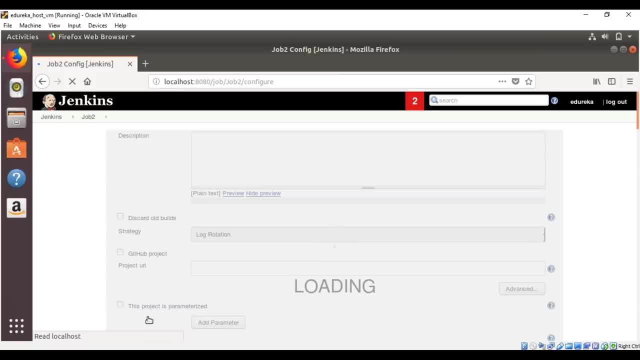 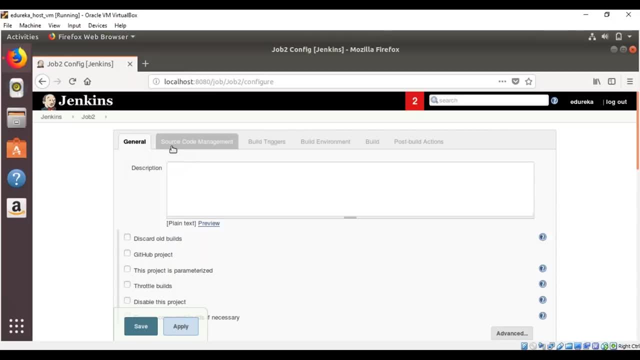 where we have to fill in all the details or whatever. we want our job to perform. So we want our job to pull the code from a GitHub repository. So let me just go to the source code management and then I'll choose the option get over here. 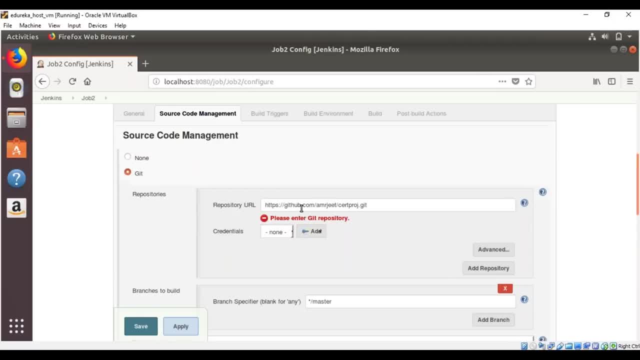 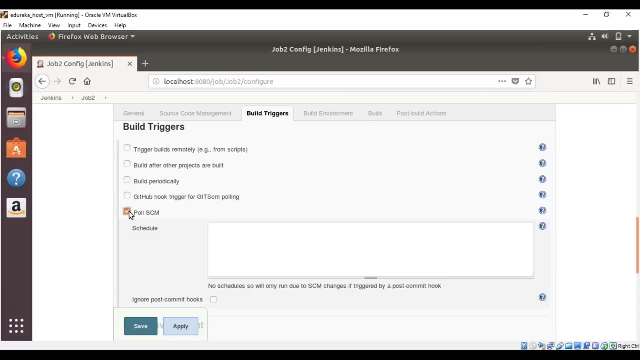 I'll mention the repositories URL. So let me just mention the repositories URL and then, if I want this build to happen again and again, I'll go to the option of build triggers and then I'll choose pole SEM. So, with this pole SEM, every time the build happens. 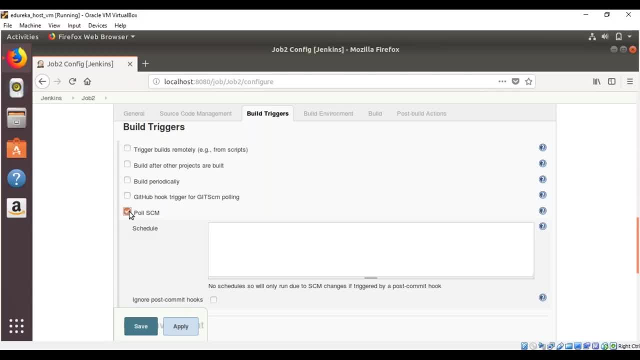 at the interval of time you mentioned. So suppose you mentioned one minute, the build will happen automatically for every one minute. If you mentioned two minutes or three minutes, the build will happen automatically at the mention time. So suppose I mention it for three minutes. 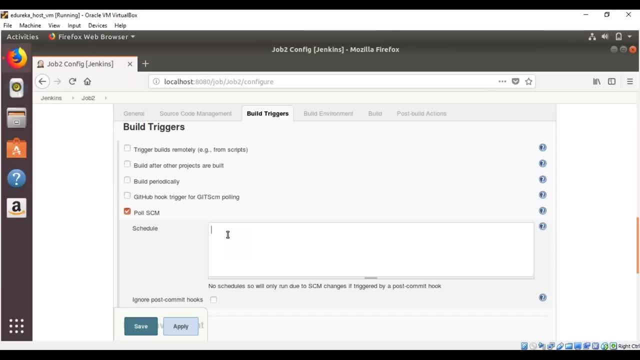 So let me just show you the build for every minute. So for that, let me just mention the time limit. So I'll mention five stars with spaces. That means it will build for every single minute. after that I'll just click on save. 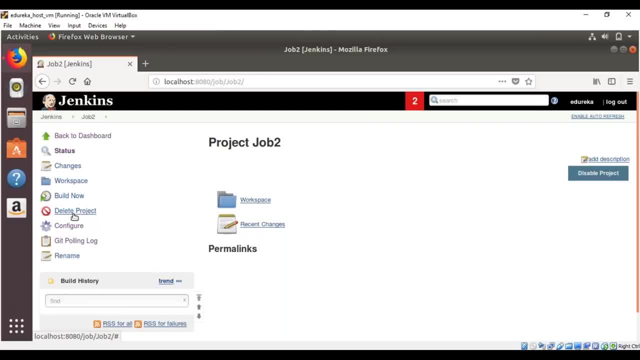 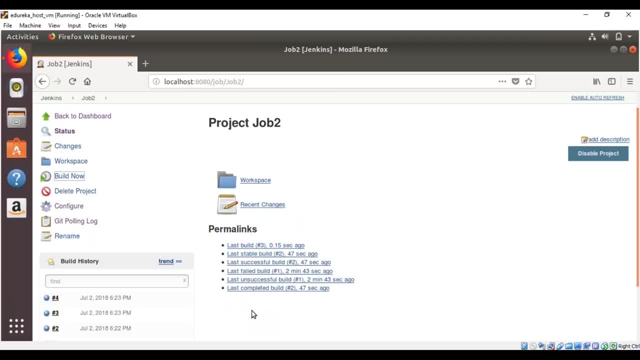 and this will be automatically applied. Now what you have to do is you just have to build this project to make it work. So you just saw that the first will happen. So, similarly, you can see that for every one minute, this build is happening, right? 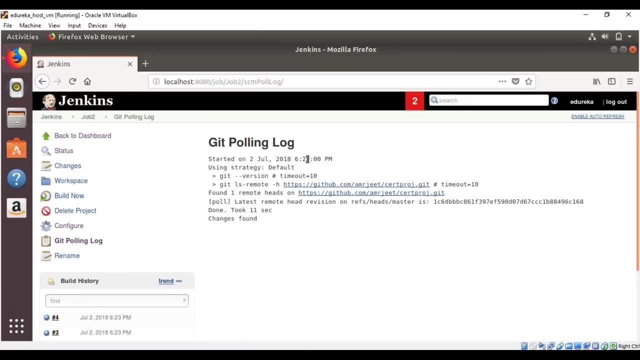 So if you just go to the guilt polling log, so you can see the latest build that just occurred, right? So you can see that it has occurred at 623.. Now let's wait for one minute and you will see that it will again occur at 624 pm. 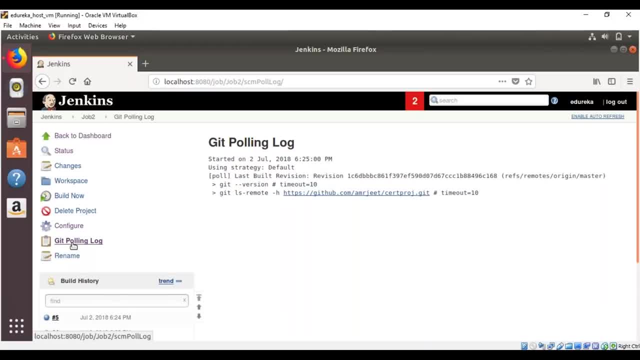 So you can see that the latest build that just occurred is again at 625 pm. That means the build is occurring every minute, right? So that's how you can automatically build your application again and again at fixed intervals of time. Now, if you have to build the Jenkins pipeline, 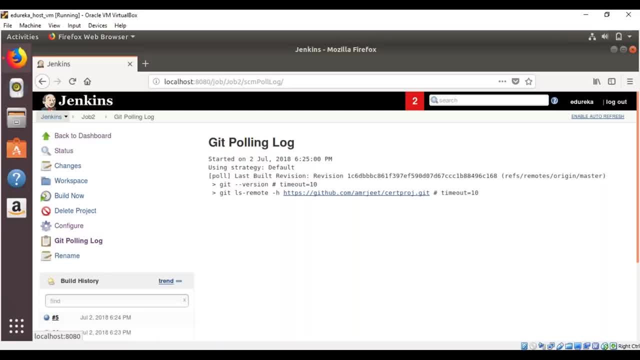 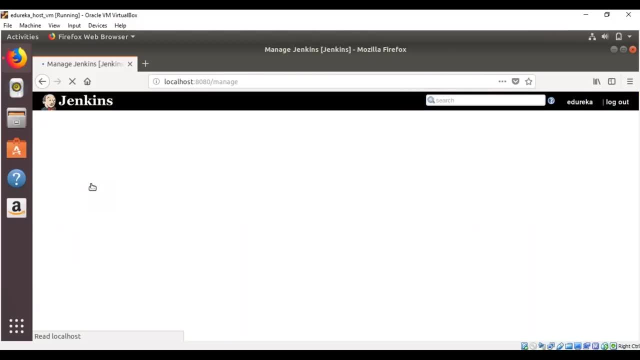 how will you build it? So for that, you have to go back to the Jenkins dashboard, and then you have to go to the option of manage Jenkins. Once you go to this option of manage Jenkins, you have to go to the option of manage plugins. 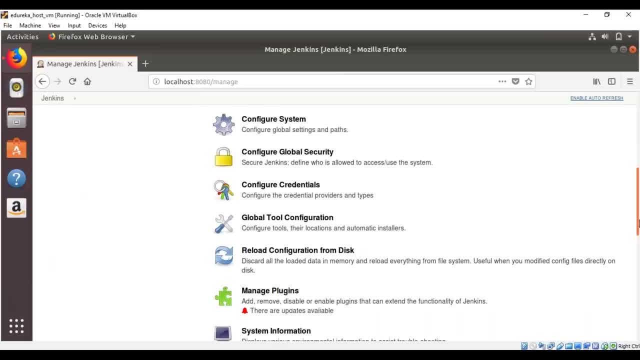 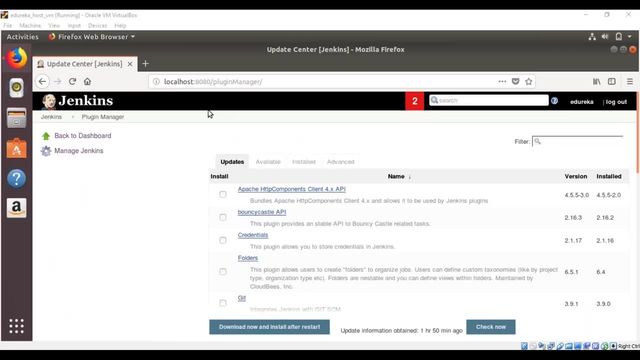 So let's just go to the option of manage plugins And then in manage plugins you can see the updated, available, installed and advanced plugins that are available for you. So to build a delivery pipeline you need the build pipeline plugin. So if you do not have it installed on your system already, 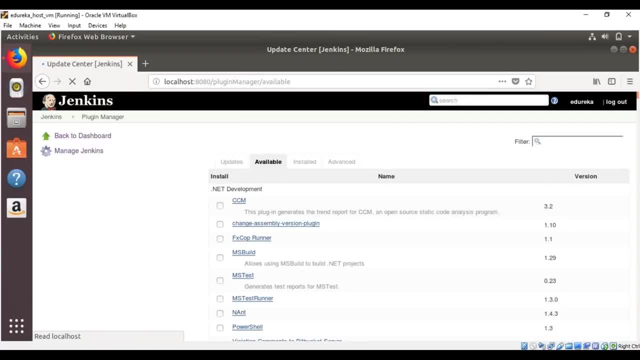 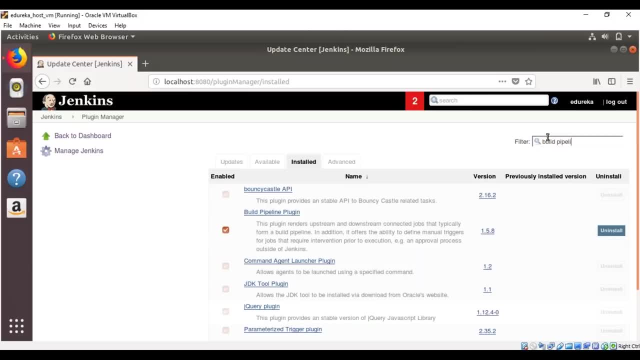 then you have to go to the available option and then search for the build pipeline plug-in here. I already have it installed in my system, So let me just show you, So you can see that it is already installed in our system, right? 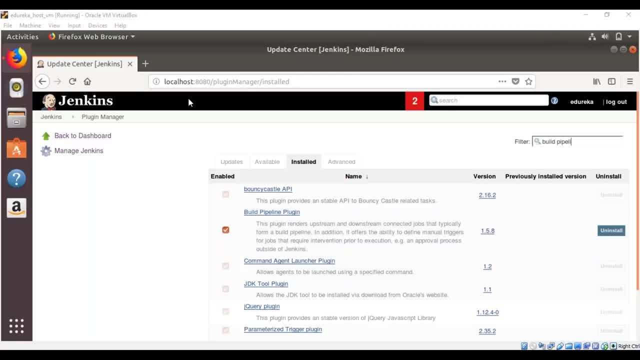 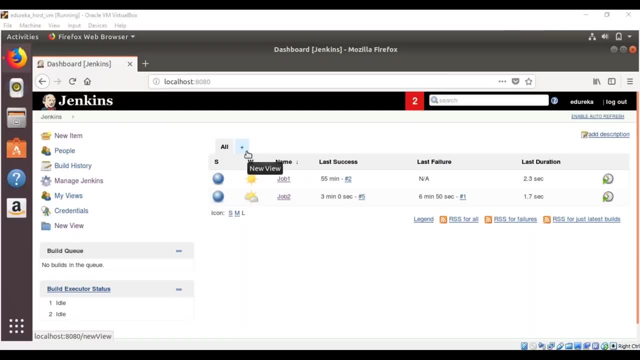 So what you have to do is you just have to go back to our Jenkins dashboard and then you have to go to this plus sign. So that is where you create a new view for the jobs. So let's just click on that And then in the view name, 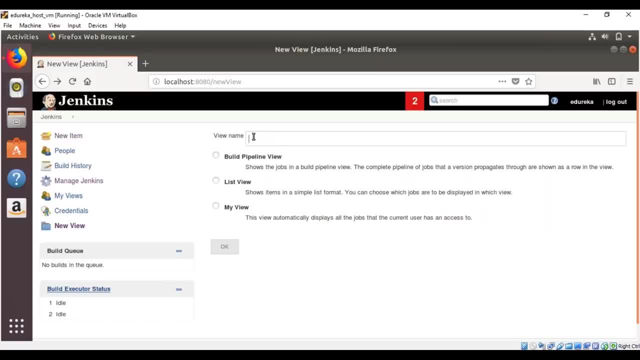 you have to mention any name that you wish to. So let's type in the view name as pipeline So, and then I'll choose the option build pipeline view. So let me click on Okay. So now you can see that your pipeline has been built. 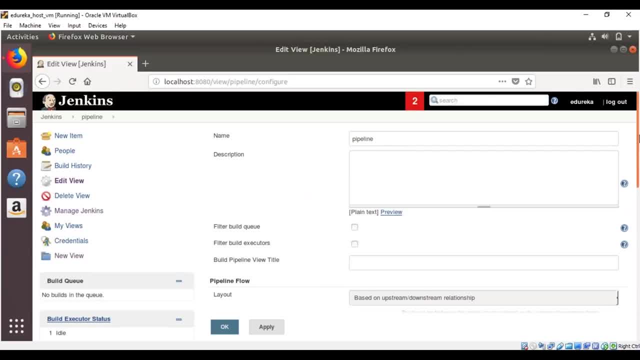 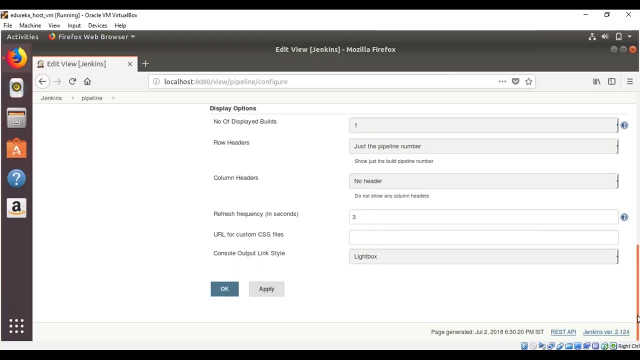 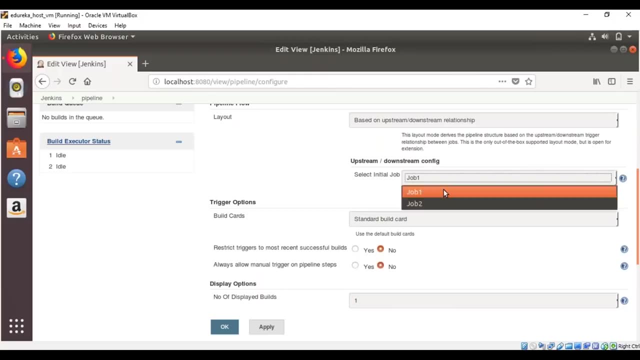 So you can see the details for your pipeline- The name is pipeline, and the layouts and the number of displayed bills for your pipeline and so on. So we have to first choose the job from which our pipeline has to start. So suppose I choose the initial job as job one and then I click on OK. 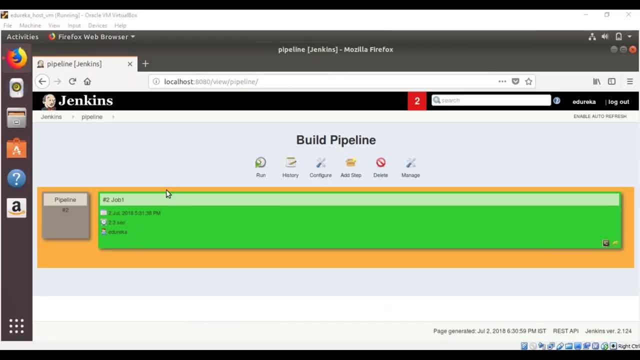 So you can see very clearly that our pipeline has the job one as our initial point and then it was built at this moment, at this time. So everybody knows at which time it was built. Now let's go back to our Jenkins dashboard, to jobs one. 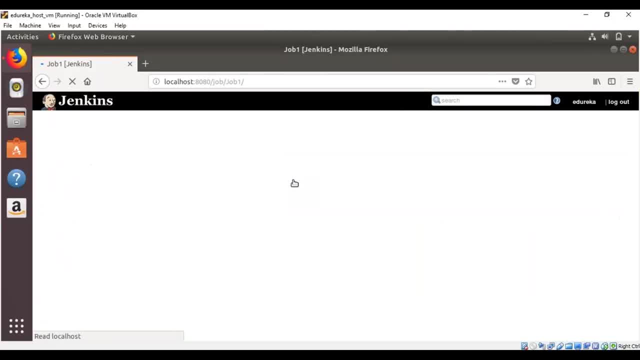 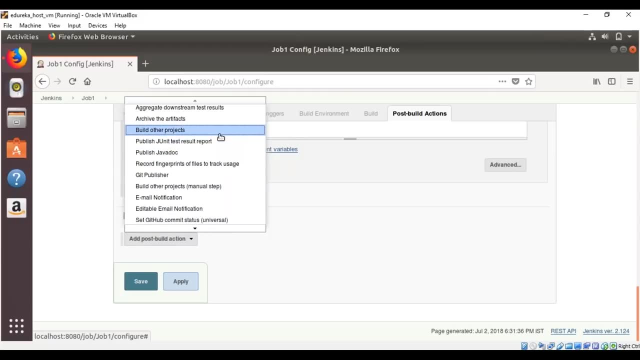 So when I go back to jobs one, we have to configure jobs one here. right, We have to configure jobs once so that it can perform post build actions. So for that we'll go to the option post build action and then over here we will choose build other projects. 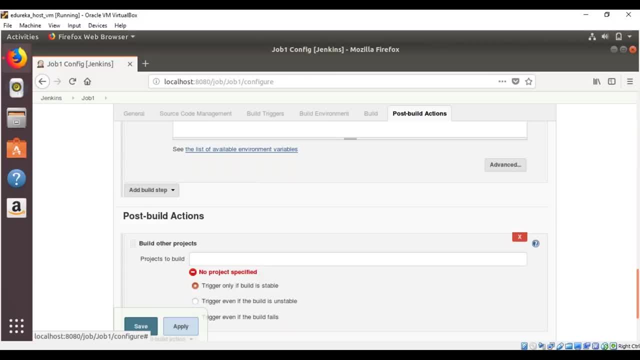 So what's happening here is you choose job one as your initial point and then you add more number of jobs So you can add like n number of jobs. So suppose, job to job, tree job for, and when the last job comes you have to choose. 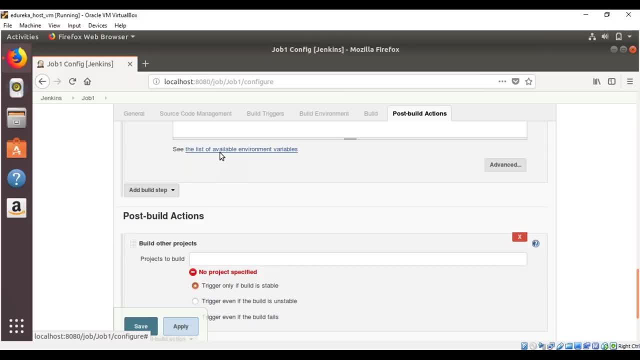 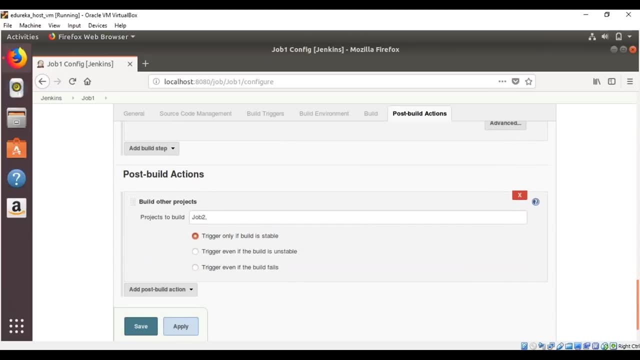 and another option so that I'll tell you soon. So we here I'll mention job to. this is the job we want after job one, and then we can choose either of the options: trigger only if build stable, if it is not stable, or even if the build fails. 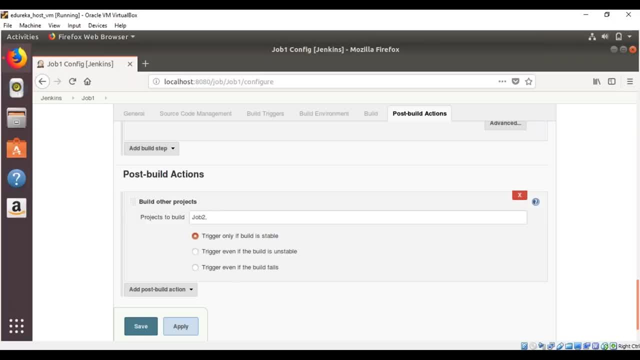 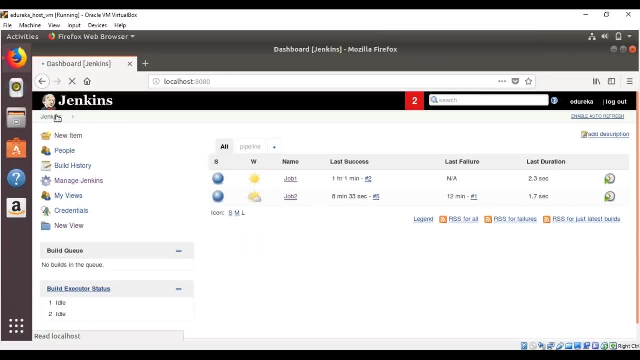 So I'm choosing the option of trigger only if the build is stable, and then I'll click on save. So once this is saved, let me go back to my Jenkins dashboard and then go to job to here. So in job to, I have to configure the build. 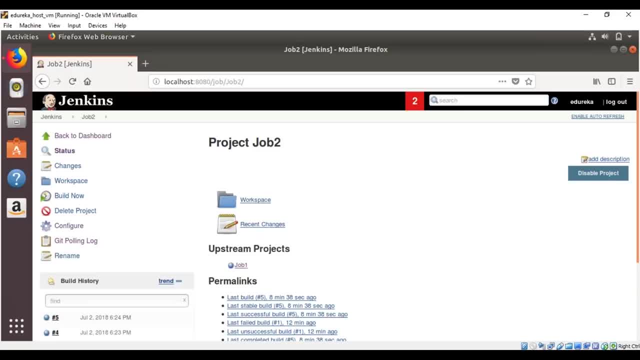 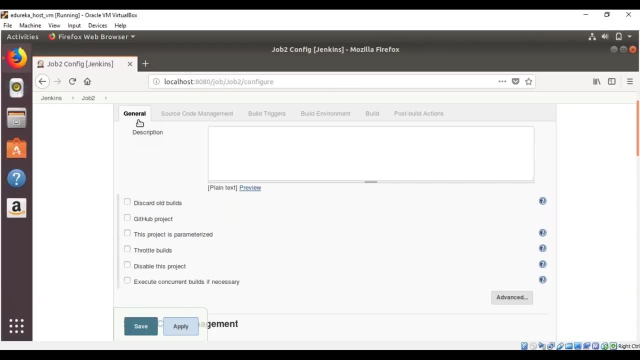 that it has to occur after the build of job one is done. So I'll go to the configure options here. So we have to configure job to in such a way that job tools build is done after job once built. So for that will go to the option of build triggers. 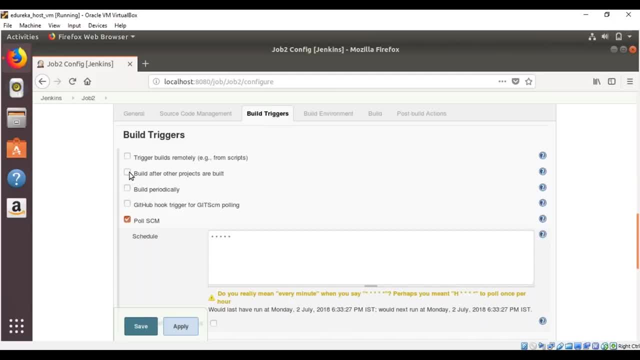 and then over here will choose build after other projects are built. So once you choose this option, we want job tools built to be done. So I'll mention job one here and then I'll click on save so you can see that this is safe. 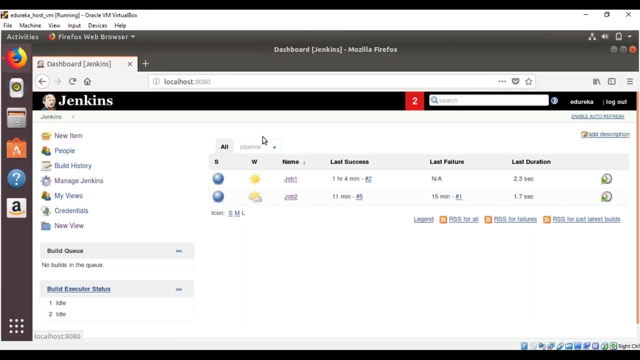 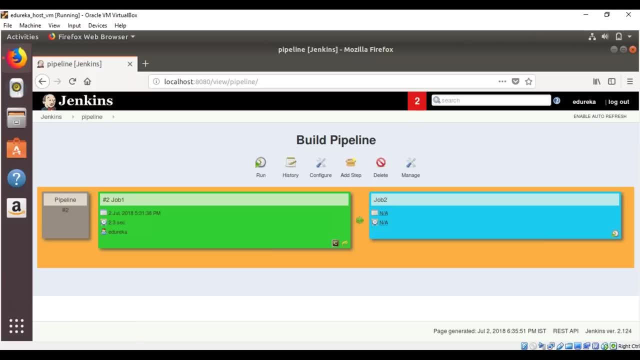 So let me go back to my Jenkins dashboard and then let me go to this option of pipeline that we just created. So this is the view that we just created for our Jenkins pipeline. Now, if we run this pipeline, what should happen is our job once build should happen. 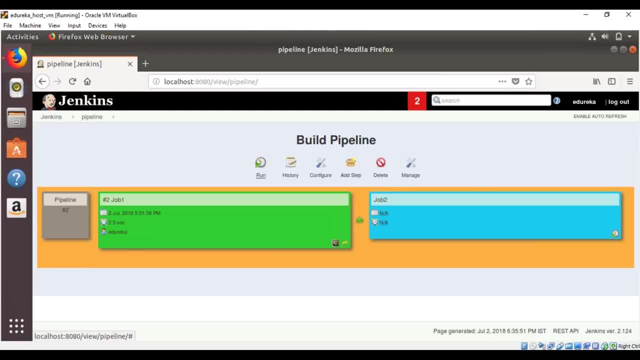 and once that build is done, job tools build should be done Right: first job once build is completed and then job tools build is completed. So let me just run this and show you so as you can see that job once build has started and then job once build has been completed after. 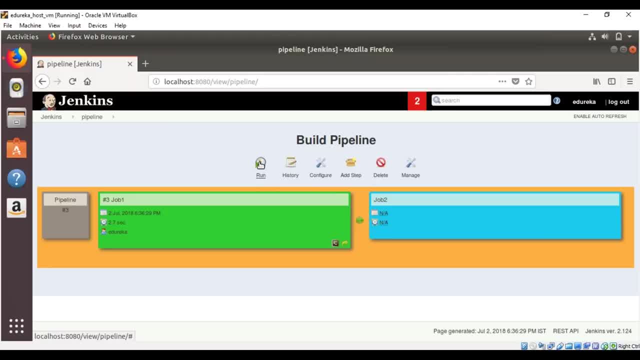 that job tools build has automatically started, and soon you will see that job tools build has also been completed, And now you can see that job tools build has also been successfully completed. So, guys, that's how you build a Jenkins delivery pipeline. So that was the end of our hands-on part. 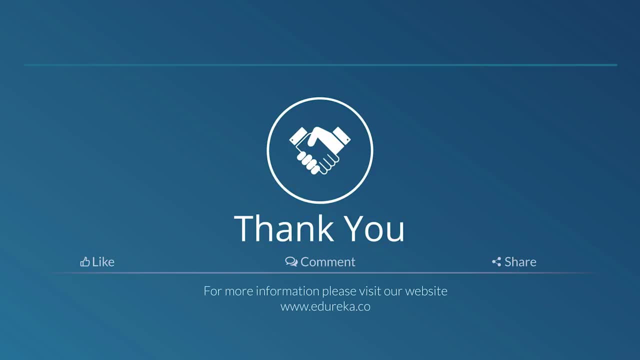 So, as you saw that agile practices and continuous integration go hand-in-hand, You can't consider your work without continuous integration. So, guys, that was continuous integration. I hope you found this video informative. Thank you and have a great day.